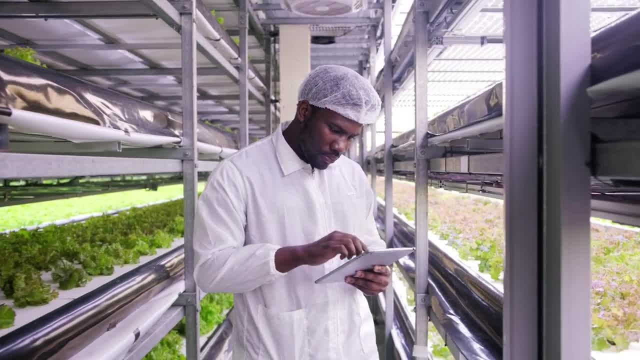 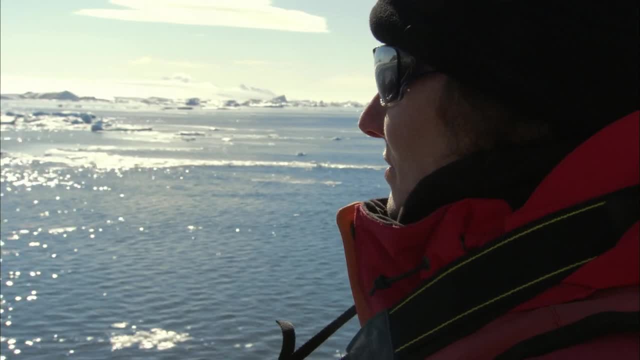 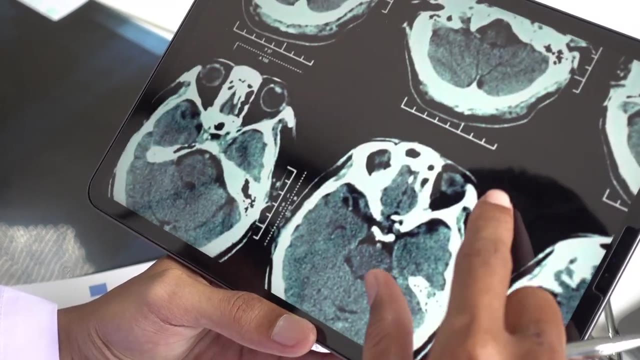 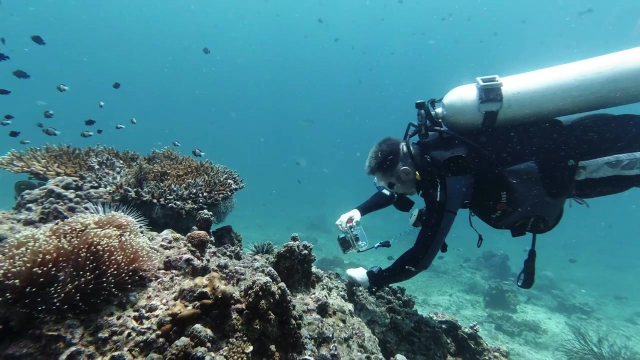 Exciting technologies developed by STEM workers include everyday conveniences like smartphones and online shopping, to large-scale game-changers such as climate change research and space exploration. to life-saving innovations like cancer treatments and Alzheimer's research. While all STEM fields involve solving problems and innovation, the work settings for STEM roles vary widely. 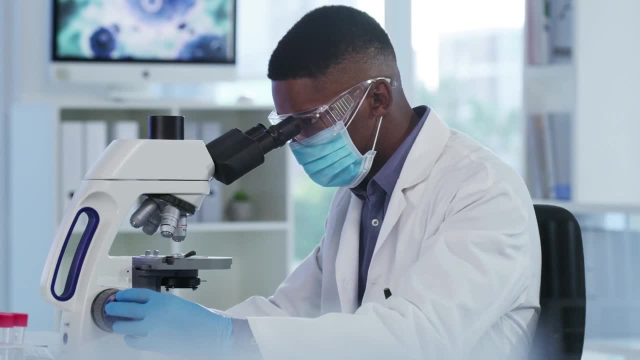 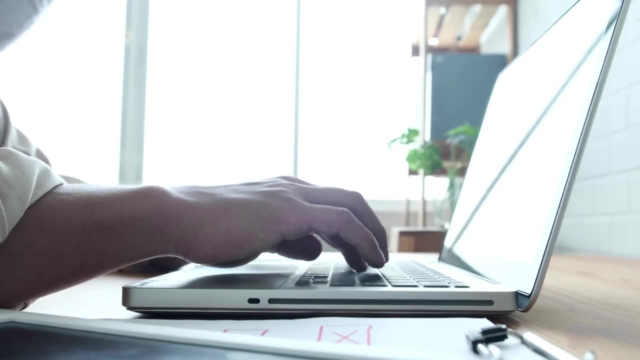 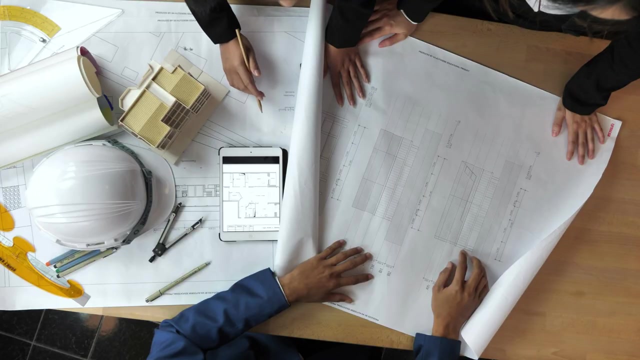 For example, research and development. scientists often work in labs to develop pharmaceuticals, biofuels and other products. while IT workers may design websites from home offices, Engineers may split their time between an office to collaborate with colleagues and work on project plans. 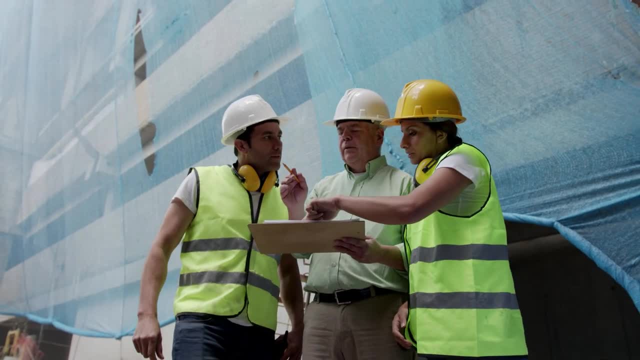 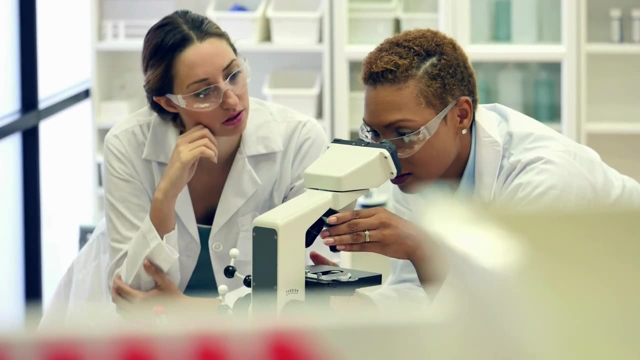 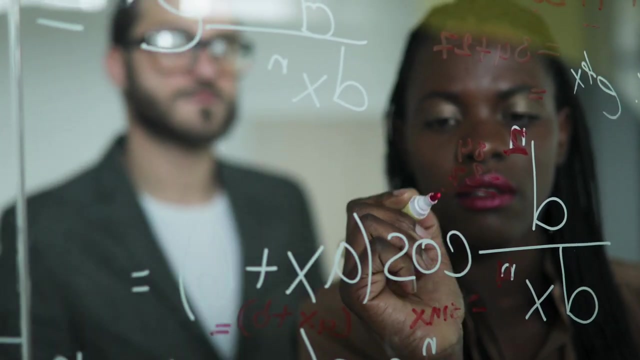 and a job site where they may supervise construction. Historically, women and people of color have been underrepresented in STEM fields, particularly in IT, math and engineering. Recently, government and industry leaders have worked to encourage more women and people of color to pursue STEM careers. 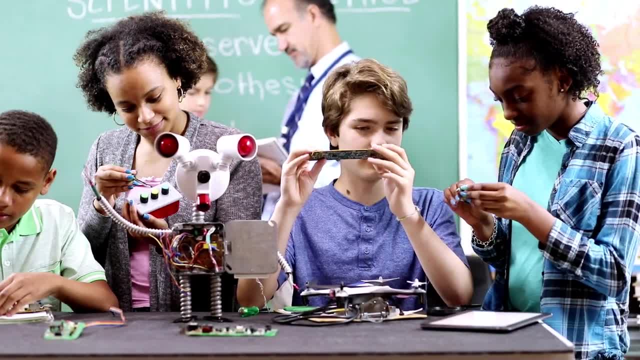 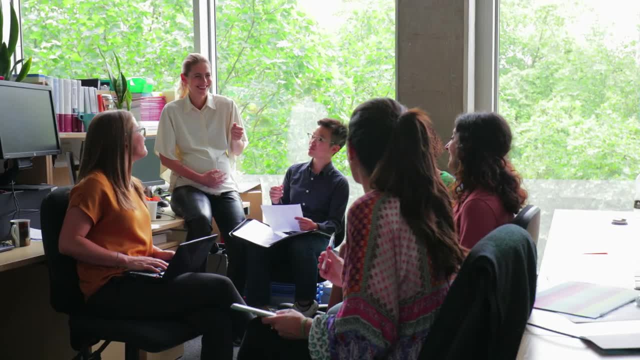 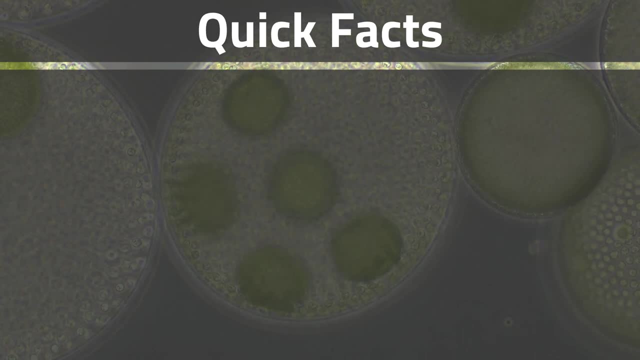 by revamping STEM education, highlighting female role models and promoting more welcoming work environments in college programs and schools. In addition to STEM programs, there are many other programs and workplaces related to STEM. Quick Facts to Know. STEM occupations currently account for nearly 10 million jobs. 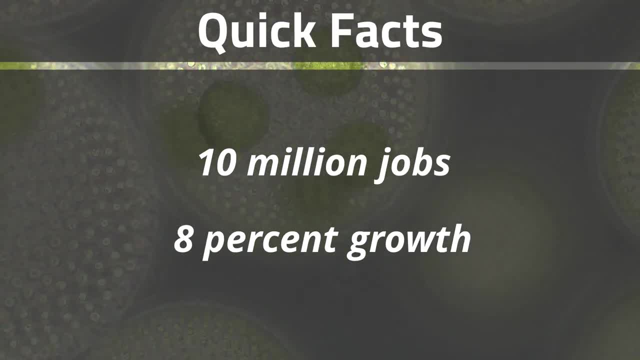 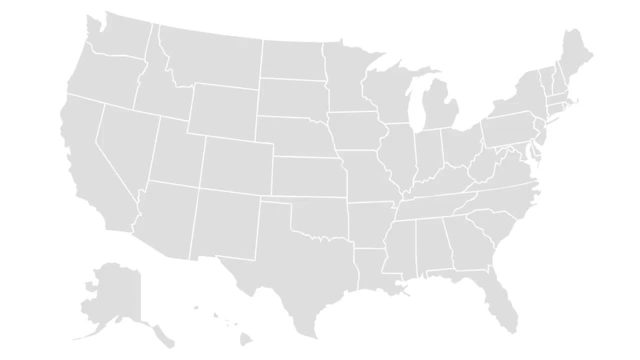 Job growth of more than 8% is projected over the next decade, adding about 800,000 jobs. STEM employment has regional centers but is expanding in new areas. Texas, New York, California and Washington employ high numbers of STEM workers. 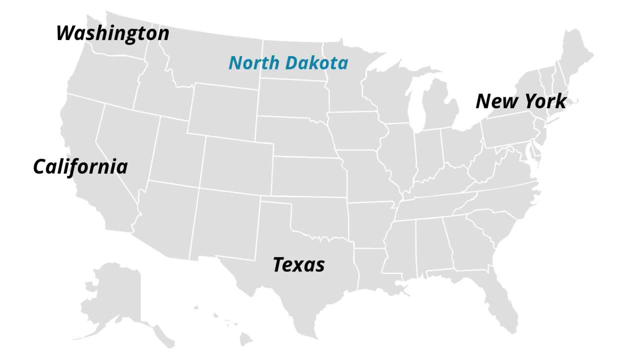 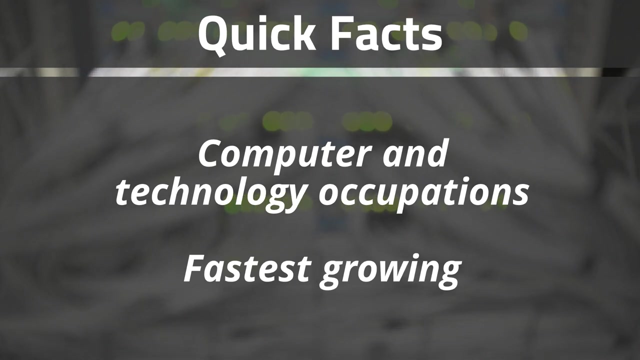 while states with lower STEM job numbers, like North Dakota, Tennessee and Georgia, have seen over 20% growth in STEM-related employment in recent years. Computer and technology-related occupations are the fastest-growing STEM fields, with an increase of more than half a million new IT jobs projected across the next 10 years. 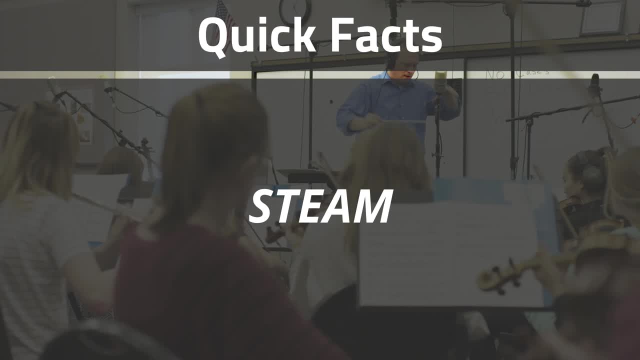 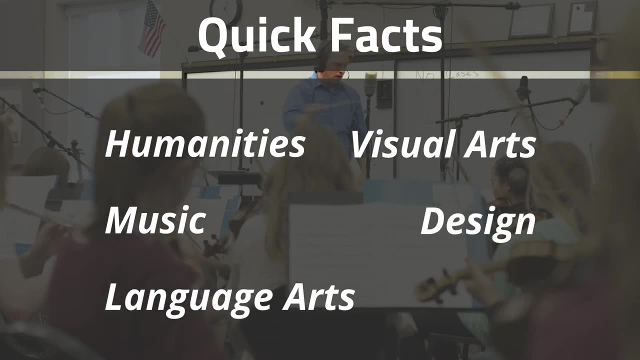 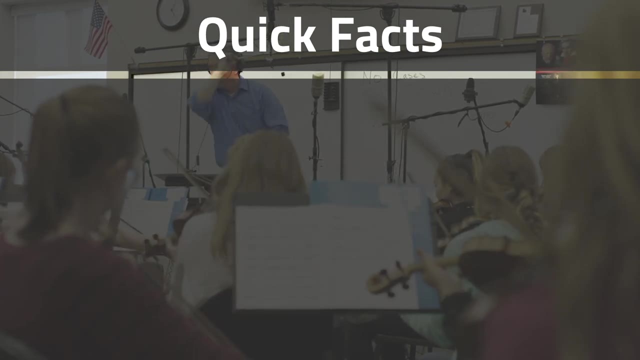 STEAM is a related global education movement that incorporates the arts, such as humanities, music, language arts, visual arts and design, into STEM. STEAM emphasizes using the creative process to investigate scientific concepts, While the job market may vary over time and location.